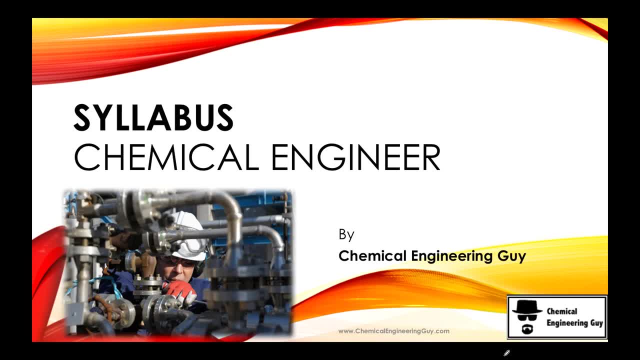 so, guys, welcome to this video series. we're going to talk about the syllabus of a chemical engineer. so, essentially, what are the courses, subjects, lab experiments and final projects, and whatever thing you can think of that you will be studying in order to get your chemical engineering degree. so I get, I do this. 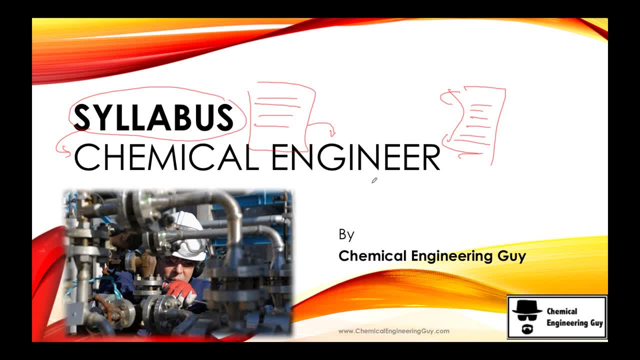 because I'm actually asked a lot of questions from you in the Facebook page or even via email. many of you are young students from high school or any other college and they asked me. you asked me: if chemical engineering is hard, what do they study? what do they work? so plenty of stuff regarding what do a chemical 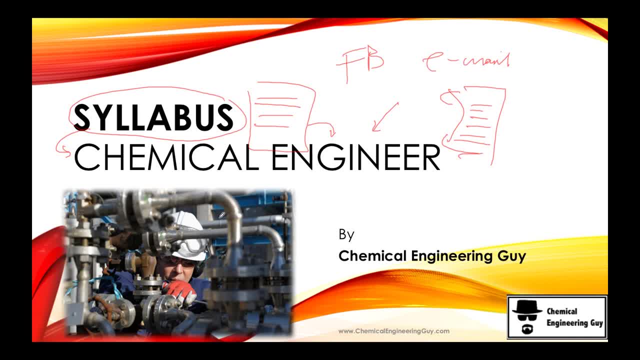 engineer do's makes, what does he work and also where, which master degrees he will be able to get, and so on. so I decided to make this video playlist in YouTube so you can check out what is the syllabus. so I'm going to explain you a little bit on what do we need to study in order to 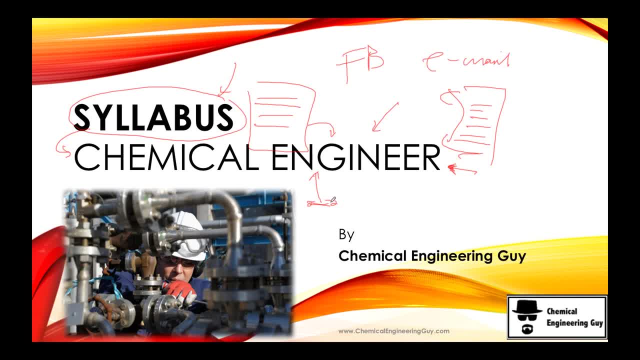 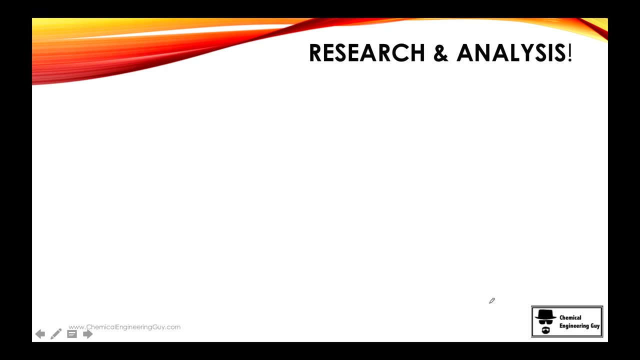 become- or, as many students will say, survive- chemical engineer. this is brought to you by me chemical engineering guy. if you want to check out more cool content, go through my website. and yeah, I did a little bit on research, informal analysis. actually, I didn't even set up a 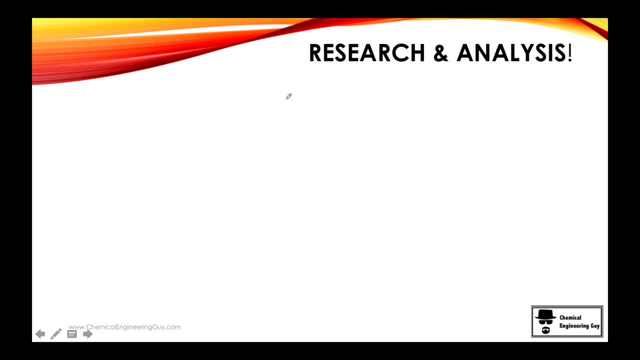 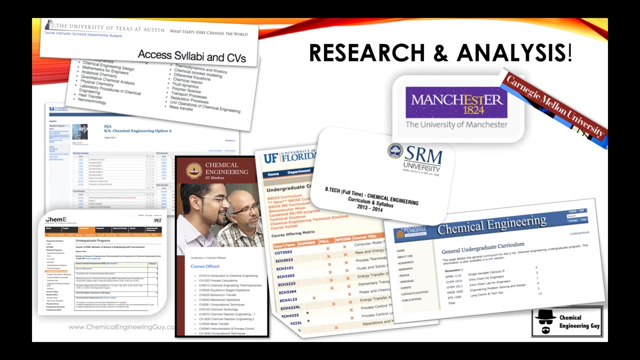 research or a methodology. I just went up online and search on Google literally wrote the words chemical engineering and syllabus or courses, subjects and so on. so I did get a lot of results. Google is almighty and yeah, essentially I got more of these, but I couldn't fit them in one single slide. 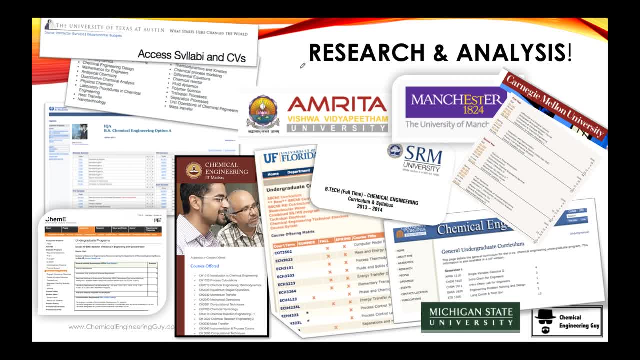 I got, let's say about 100%. I will say 60% was USA University, so you can check this here: University of Texas at Austin, MIT, University of Florida, University of Virginia- which I didn't know it existed- MSU Carnegie Mellon. then about 15% was. 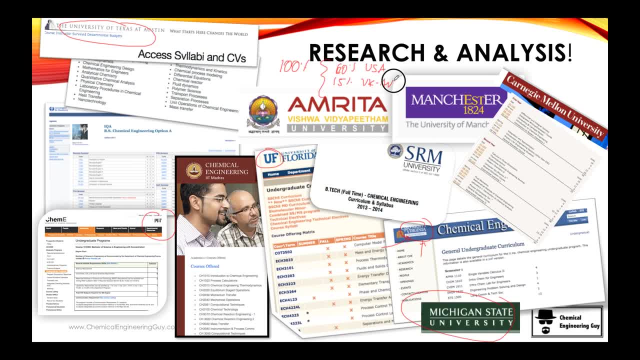 either UK or Australia or South Africa, which I think is also, I will say, Canada, all the Commonwealth countries and the other, I don't know. it's like 25%, it's really all around the world. so, for example, India also is my home or alma mater University. take the. 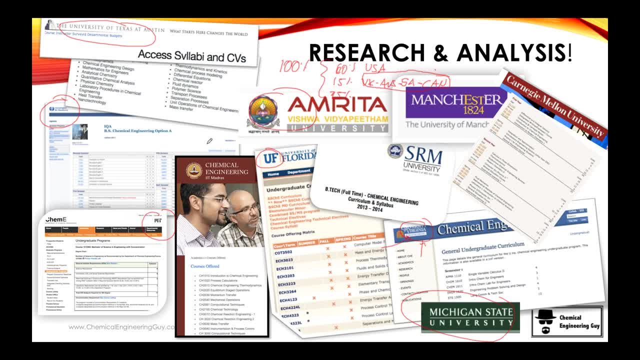 Monterey from Mexico. I also checked out in Chile, Argentina, some Egyptian universities, also some in Saudi Arabia, which they had a lot, it makes sense, because they have a lot of oil. also, I checked plenty of German universities which I will say they are very, very, let's say they have a lot of. 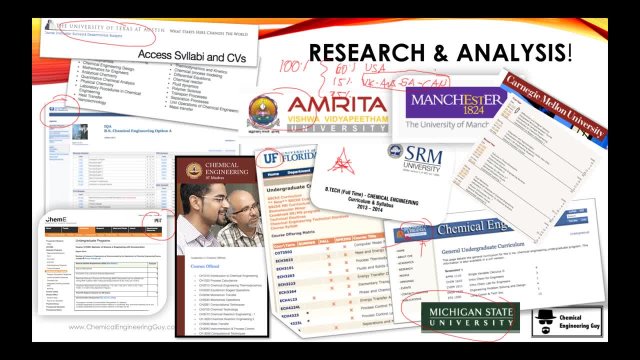 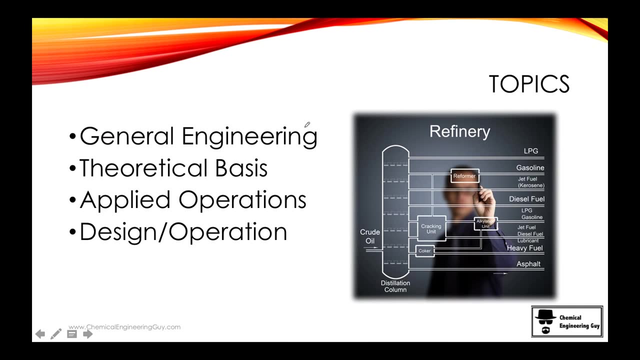 universities regarding chemical engineering and also French ones. so I did in general, I tried to go and check out for the whole world, or at least the world that typically goes into chemical engineering, and, yeah, I was wondering on if we actually study the same around the world. so we have- this is sorry that good drawing. so this is Europe, Africa, Middle. 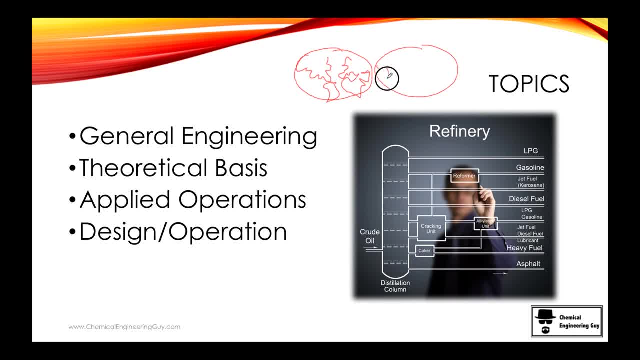 East and maybe this is India and Thailand and all those countries, Japan, beautiful Korea, Australia. so I did check out if we actually check or study the same things. so in the USA- or at least this was my guess- in the USA they see a lot of economics and maybe 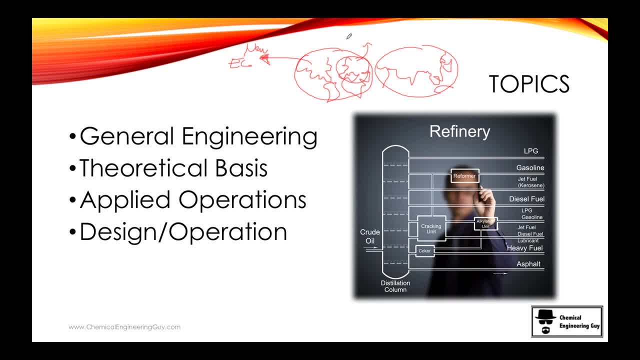 new technologies in Europe? I will say they have more about on the environment in Asia. sorry, Asia here, China maybe, or Japan. Japan, I will say they have technology. I will say India, you have a lot of computer related process engineering or maybe simulations, modeling, software modeling and so. 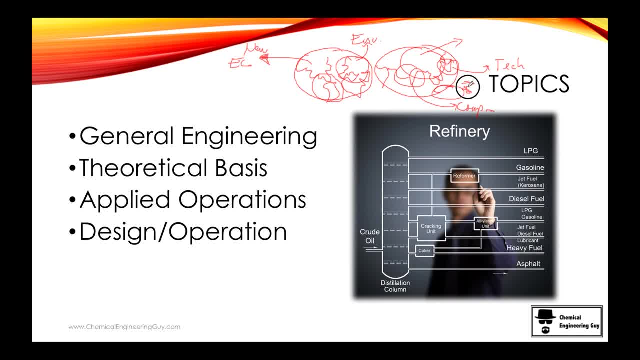 Australia didn't even have a clue, but I did in Australia. I did not even have a clue. I don't know what they are good for. sorry for you guys, but I don't know if there's even petroleum there. I think there is, and for Africa and Middle East, well, I thought about petroleum, petrochemicals and stuff. so the good thing is that, even though we are in a huge global continent or world, I could divide into four regions or, let's say, blocks. topics: the chemical engineer, bachelor. 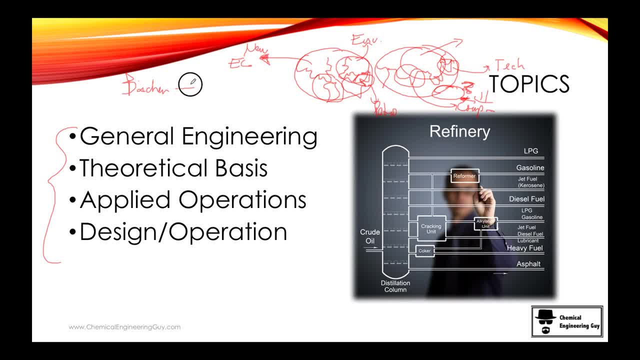 when I speak about bachelor, I mean about when you convert from high school to engineer. so the good thing is that we are actually starting more or less the same. things like unit operations and theoretical bases are similar. we eventually end up doing some projects on plant design and so on, so that's good. the other thing I wanted to show you guys is that actually 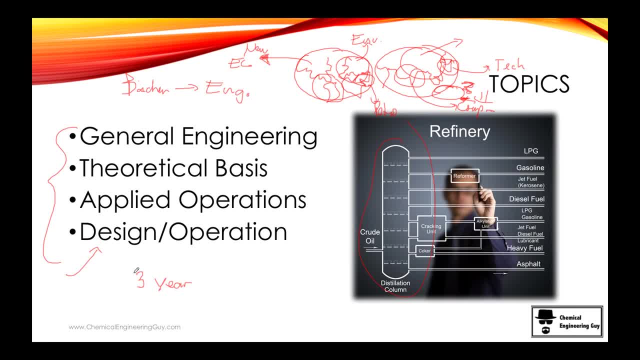 I three years, so I checked out how long do you need to study in order to convert into an engineer. so the average was about three years to four years, with, of course, its exceptions, but the mainly. I would say 80% is about something around four years and the 20% something around three years. so yeah, of course, maybe there are some places you need five years and maybe two years, but in general what I saw- the number of semester courses or trimesters and so on- 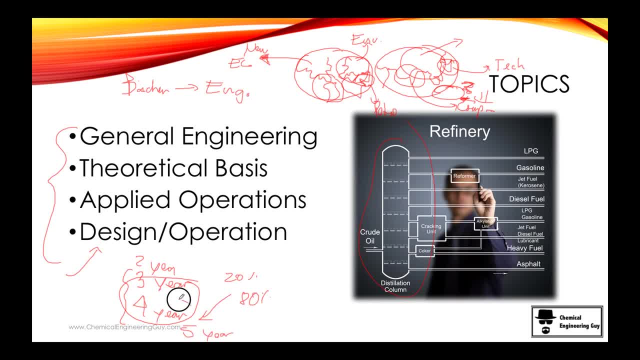 was about three to four years. so I'm going to, since we have 80% of this, I'm going to pay more attention into the four years and I got these blocks right here. so you can see there are four blocks: the first block, which is roughly translated to the first year of your, let's say, training, then the second year, third year and final year. of course, if you have a three-year program, well, you will have the same blocks, just differently set. 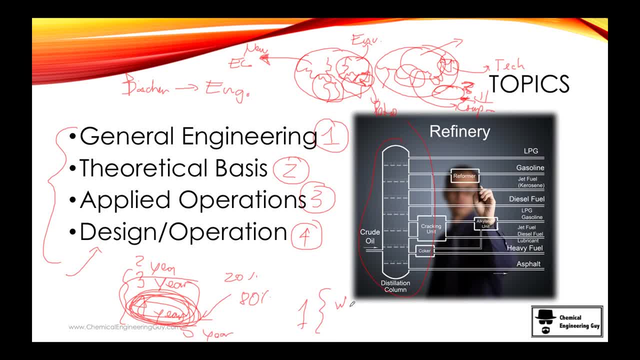 so recall that one year has two semesters. I would say winter semester and summer semester, or spring and autumn, I don't know how you divide them. so well, the first thing I wanted to show you is that we all start with general engineering. we study a little bit on math, a little bit on sciences, a little bit introduction to our engineering fields- environment and so on- and of course math. 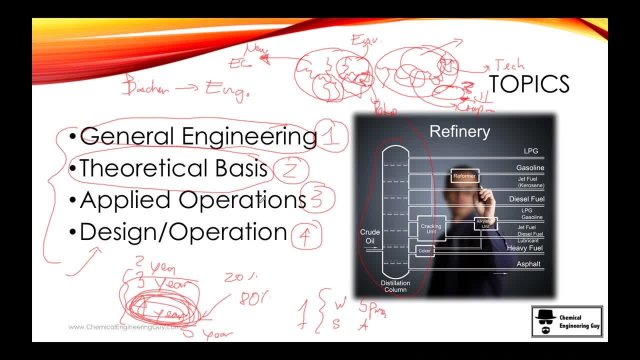 then eventually we go and check out for the theoretical basis. but we're starting to study a little bit more on the thermodynamics, on transport phenomena, mass balances and energy balances, but still we don't have the ability to create unit operations, which is in the third year. in third year you will see a lot of, let's say, heat transfer, momentum transport, fluid dynamics, mass separation, mass transfer and so on, and you will be able to do these beautiful buildings right here. 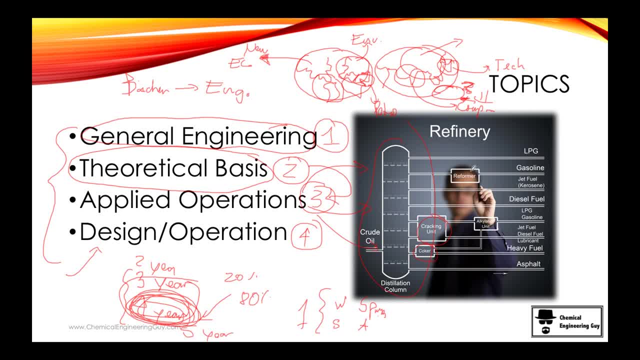 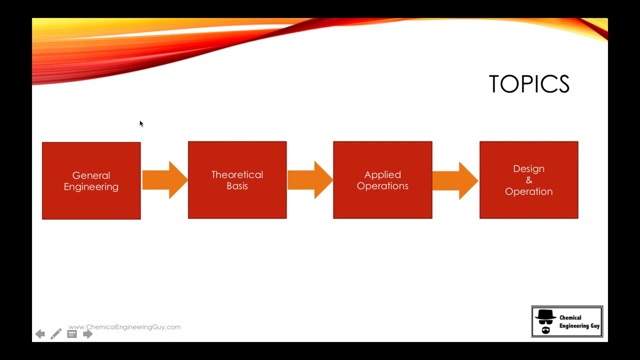 like a distillation or cracking unit, cooker, reformer, reactors and so on. eventually, once you actually know a little bit on the basis and about the unit operations, you eventually create your chemical plant to produce a product which you will want to sell, probably. so this is what I wanted to show you guys. I also read a lot on the requisites, so, for instance, 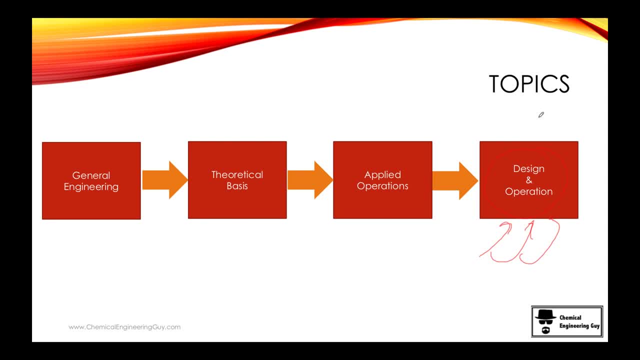 all the countries, I checked all the universities, they will, let's say, if you want to study plant design, you cannot just go there and sign up. you need to study unit operations, which are essentially heat, mass, momentum and reactors. and in order to know about, let's say, reactors, you will need to have a little bit of insight on the chemistry of reactions, kinetic models, organic chemistry maybe, and so on. 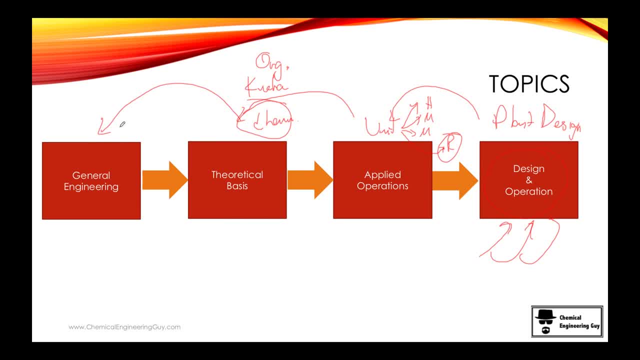 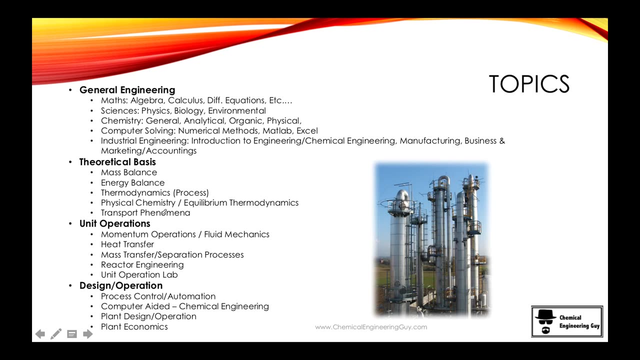 and in order to know a little bit on this, you will need to know the general stuff like math, models, chemistry and so on, so that's a good thing. all the places or universities I checked they have prerequisites, which is, I think, very important, and what I'm going to do in the next or following videos is essentially just break up all these blocks. they are the same topics I showed you before, but right now it's 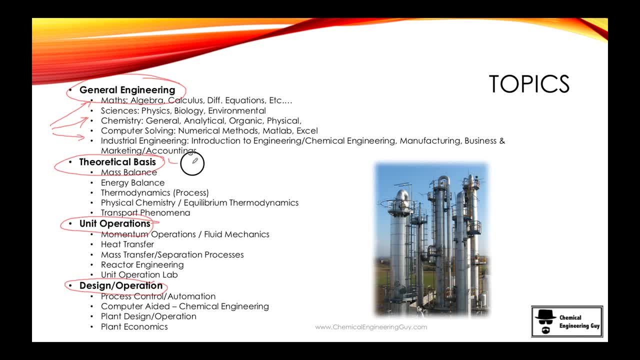 let's say, into assignments. so what I want to cover the most is this part right here which is the actual chemical engineer stuff. this is general engineering, what every engineer should know, or at least so. for instance, algebra, calculus, differential equations. you should be sure that if you're talking with an engineer, you should like assume that he knows about equations and how to solve them, and so on. 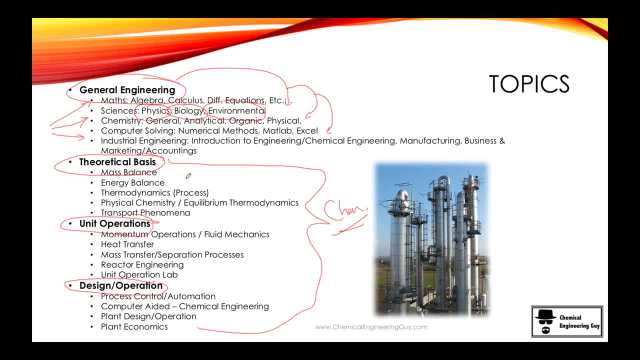 a little bit on physics, biology. this right here is pretty special for the chemical engineer. so you will expect that one engineer knows the basics about engineering, so for instance a chemical equation and all that. but of course we go a little bit deeper than normal engineers. but that's another thing. 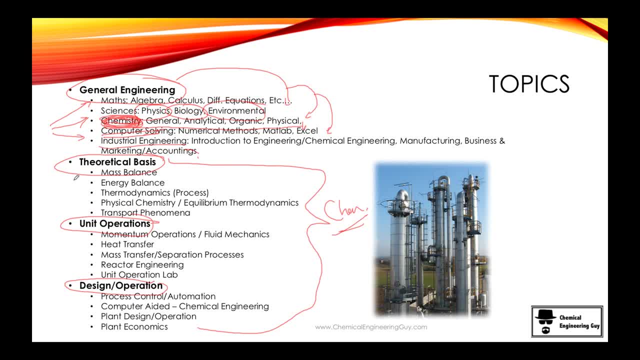 and computer solving, industrial engineering and so on, and then I will think this is the actual first block where you will see if chemical engineering, engineering, is for you. so maybe you love maths, you love sciences, you love computers, but then you go. 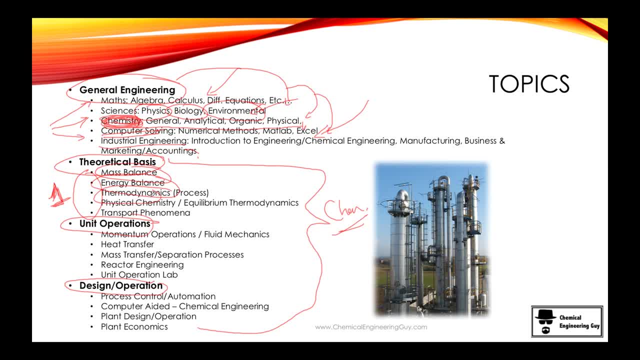 to the mass balance course, energy courses, thermodynamics. and then you say this: i don't, i'm not into that, i'm more about the computer software. or maybe you are more into mechanical engineering. you're you don't like that much maybe balancing a process you prefer. 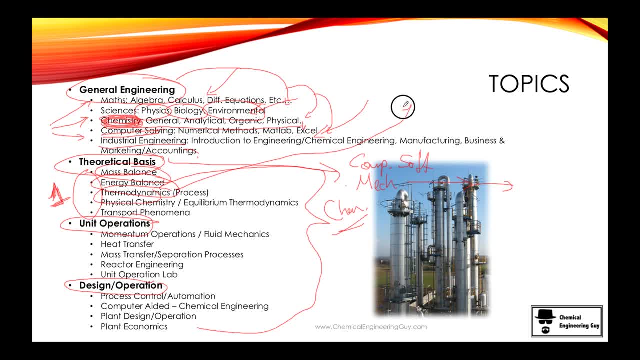 the material. so maybe you say: fuck this, i'm going for civil engineering, i prefer buildings because yes, as i tell you before, i'm good algebra, calculus, differential equations, a little bit of sciences. i do like chemistry, but more about materials used in the construction. so i think 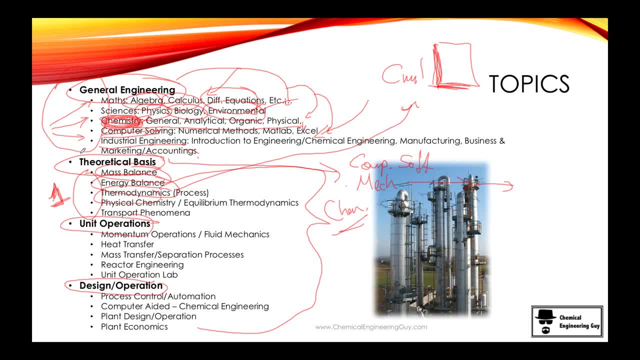 the first, let's say, this one right here is just to say that you like engineering. so if you're in the first year- which is this one right here- general engineering, and you don't like it? well, this may be because, oh fuck, i don't like math, so i'm into art. 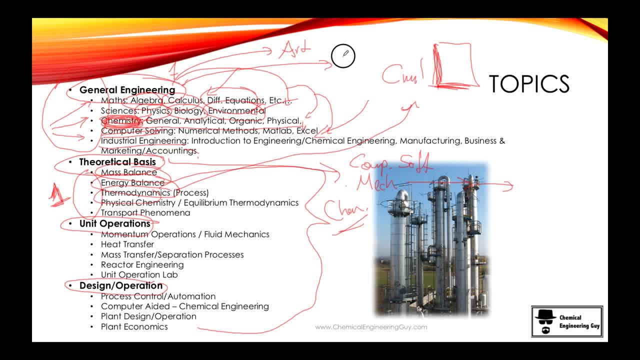 or maybe you say i don't like physics so i'd rather become a doctor. or you say i'm not into computers so i will go, and maybe i don't know- study literature. so the first year is you are about engineering. the second year, which is the theoretical basis, i will 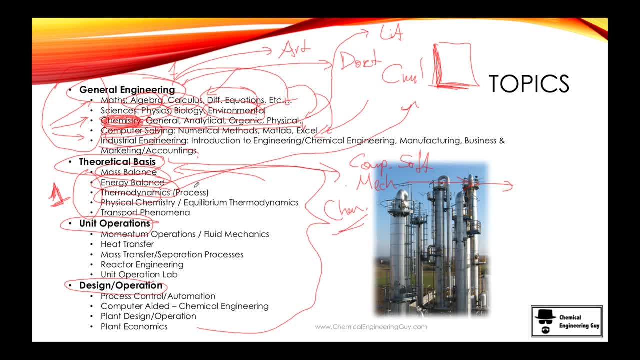 say you are into process engineering- maybe mechanical engineering, process engineering, petroleum engineering, chemical engineering, anything related to processes- and eventually i would say that in the third year right here, this is literally all about process engineering. so i think if you make it up to here you will probably stick to it, because you this is pretty similar to this right here.